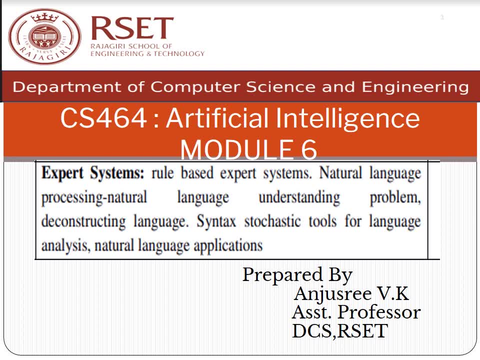 Hello everyone, Welcome to the online lectures of Rajagiri School of Engineering and Technology. I am Anjusri VK, working as Assistant Professor in Department of Computer Science and Engineering, Rajagiri School of Engineering and Technology. Today I will be handling the course CS464- Artificial Intelligence, Module 6.. The Module 6 of Artificial Intelligence covers the following topics: Expert Systems, Rule Based Expert Systems, Natural Language Processing, Natural Language Understanding, Problem Deconstructing Language Syntax, Stochastic Tools for Language Analysis and, finally, Natural Language Application. 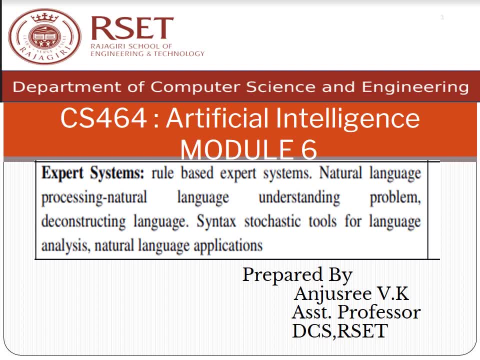 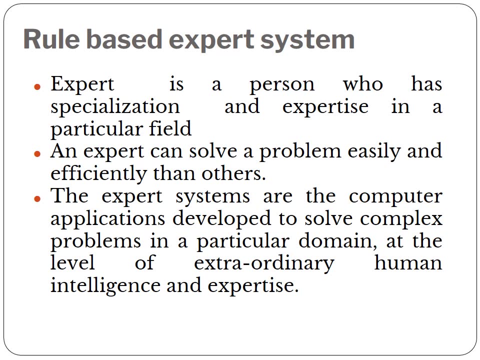 Today, in this session, I will be concentrating on AI Expert Systems and Rule Based Expert Systems. So let's check: what are the details of this Expert Systems? What is a Rule Based Expert System? So today, the most important areas of AI are centered around Knowledge Engineering in general and Expert Systems in particular. 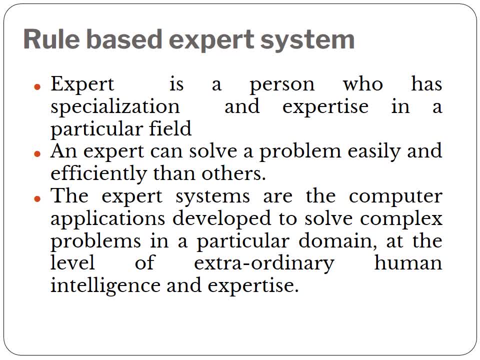 Considerable amount of success that Expert Systems have gained in the areas mentioned during the past few years. There are many examples of Expert Systems that have led to substantial amount of interest in variety of fields, such as Batch Plan Management, Optimal Routing, Fault Diagnosis, Optimal Portfolio selection, etc. 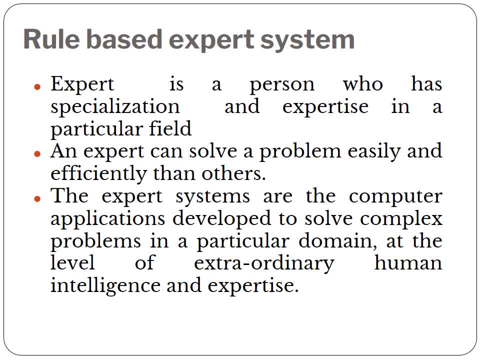 So what is an Expert and Expert Systems? An expert is a person who has specialization and expertise in a particular field. It means an expert has knowledge and skills which most of the other people do not have. An expert can have a lot of expertise and expertise in the field, but it can also be a problem maker. 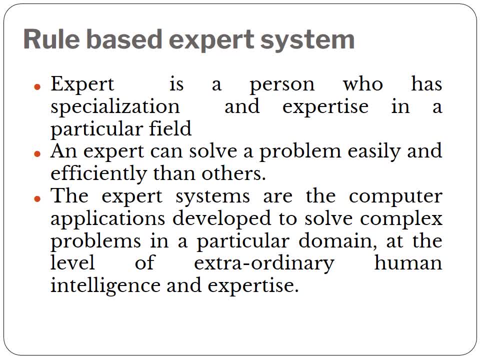 So what are Expert Systems and looking for in Expert Systems? An expert can have a lot of expertise in the field, but it can also be a problem maker. An expert can have a lot of expertise in the field, but it can also be a problem maker. 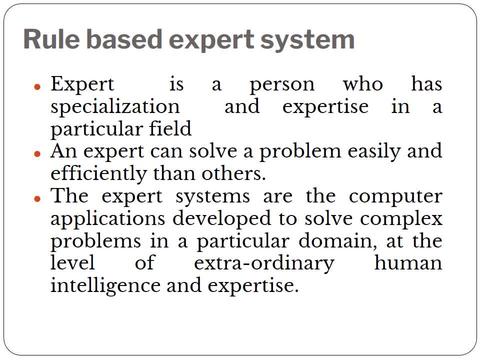 but can solve a problem much easily and much efficiently than others who cannot solve that problem. For example, if you are considering an eye surgeon, he will operate and solve the problem related to eye in a much professional and efficient way compared to a normal person, only because an eye surgeon is an expert in his field. 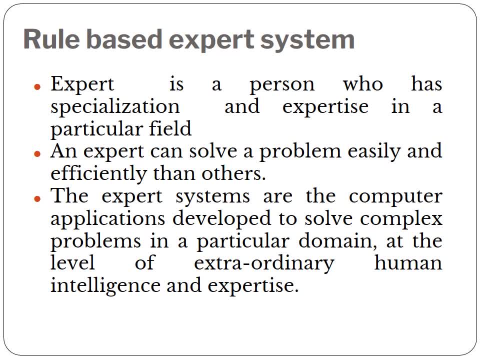 An expert system is also something which acts as an expert of a particular field, just like human expert. So it means an expert system is nothing but a computer program that acts intelligently and solves the problem in the same manner in which a human expert will. 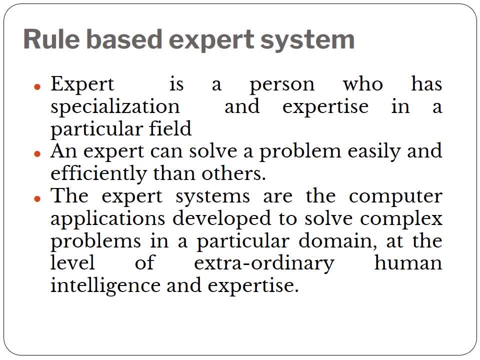 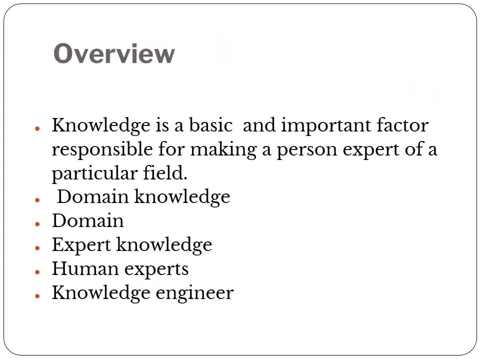 So we can also define an expert system as an expert system where the computer applications developed to solve complex problems in a particular field. So an expert system is a particular domain at the level of extraordinary human intelligence and expertise. So the overview of expert system. 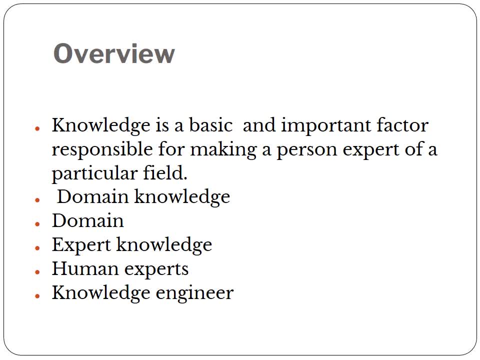 So, if you are considering a doctor, he is able to diagnose and cure a disease because he possesses knowledge about medicine. Similarly, if you are considering a geologist who is able to discover mineral deposit because he possesses deep knowledge about geology, Doctors and geologists are considered experts. 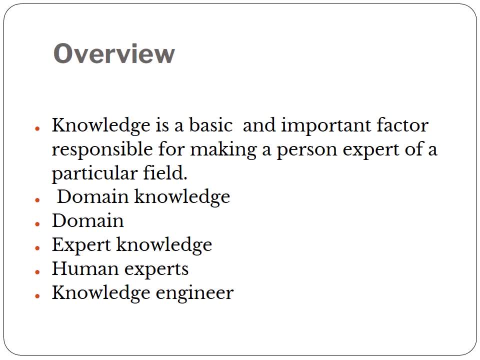 They are called experts of their respective areas. Experts possess deep knowledge about their area. They acquire this knowledge from books, magazines, journals, etc. and through experience they gain from working over the years in a particular field. Hence, it should be understood that knowledge is basic and most important factor responsible for making a person expert of a particular field. 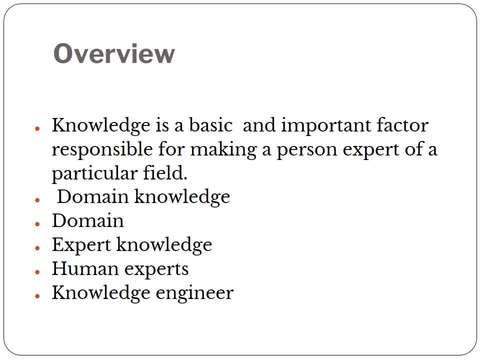 The knowledge of a specific field possessed by an expert of that field is called domain knowledge. The job of experts is to solve any problem related to their area of interest. The information related to the problem is called problem area or domain For solving any problem. first step is to identify the domain of problem to be solved. 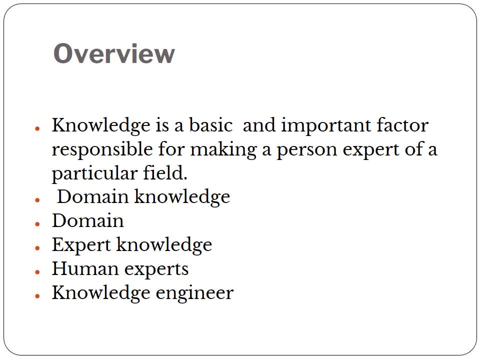 After this, the problem is passed to an expert who possess required information. The expert must have a certain amount of knowledge or expertise about that particular domain. Expert knowledge is a combination of theoretical understanding of a problem and a collection of heuristic problem solving techniques. 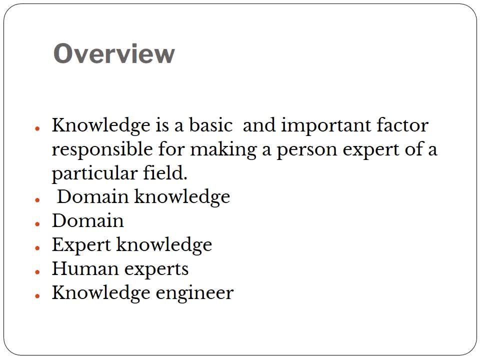 An expert applies both of these for solving a particular problem. Expert systems would primarily require deep knowledge of a particular area. This knowledge is acquired from human experts, and coding of the same is done into a form That is applicable by a computer to solve a problem of a particular domain. 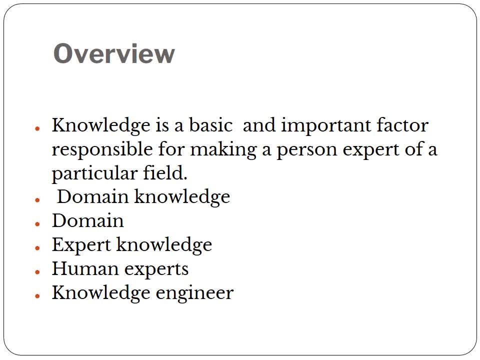 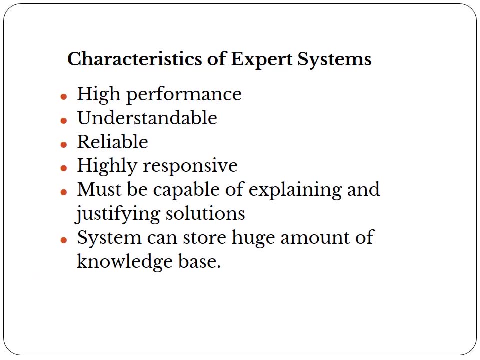 So there is a knowledge engineer then codes this knowledge explicitly in knowledge base and use the same for developing a computer program that is both effective and intelligent in its behavior. So that is all about the overview of the expert system. So next is the characteristics of expert system. 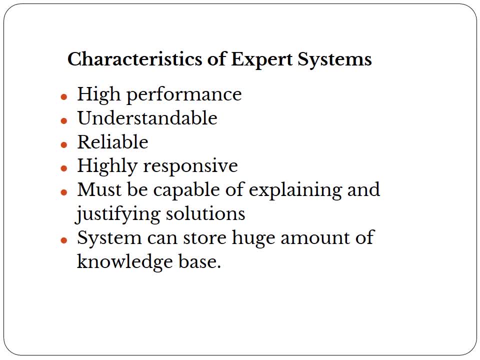 So expert systems are constructed to assist and replace human experts from intricate problem domains for achieving efficiency and economy in problem solving techniques. So an expert system normally should possess the following features. First one is high performance. So if you are taking consideration of the performance of an expert system, it must match that of a human expert. 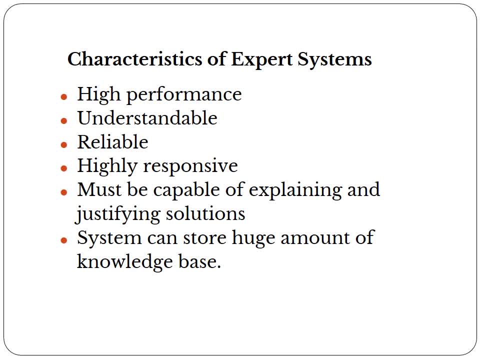 The solution provided by the system of a given problem should be of high quality. This should differentiate the expert system from other computer programs, mathematical modeling or computer animation. The next is understandable. The system should be able to solve the problem by use of more and more heuristic knowledge or any other type of knowledge. 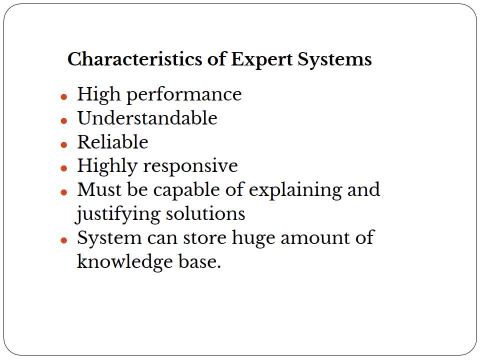 This ability makes them comparable with human experts. The fourth, or the third one is the reliability. The expert system must exhibit high level performance in terms of speed and reliability in order to be a useful tool. It should not be prone to crashes and should be able to give steady and consistent performance. 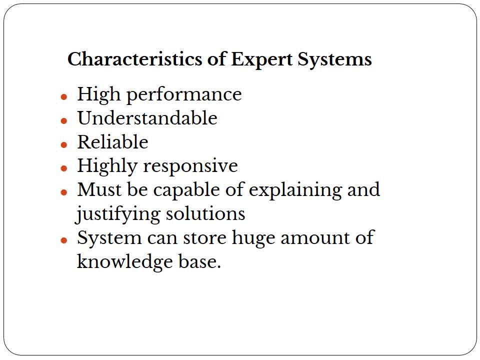 The next one is highly responsive. The response time of the system should be adequate. The system should produce results in reasonable amount of time, comparable or better than that of a human expert. The next is the expert system must be capable. The expert system must be capable of explaining and justifying solutions or recommendations in order to convince the user that its reasoning is correct. 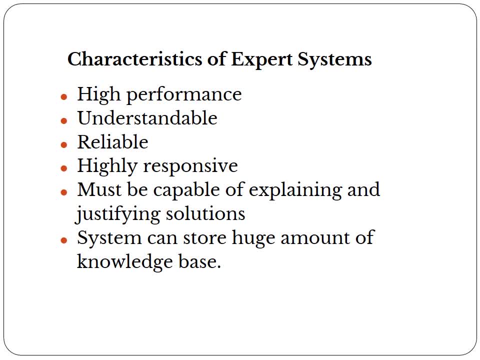 The last one is the system can store huge amount of knowledge base. Hence it should possess desired level of flexibility, so that addition, correction, deletion and modification to the knowledge base can be done as and when required to improve the performance of the system. 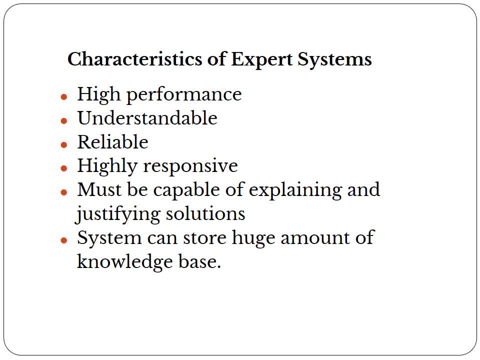 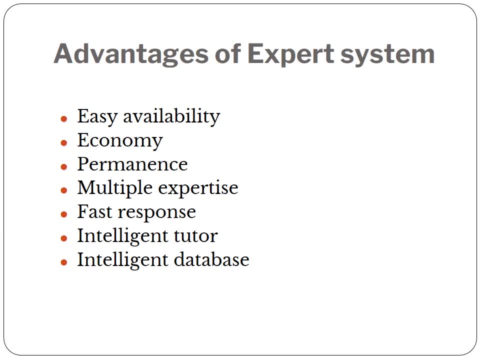 So that's all about the characteristics of expert system. So next is the advantages of expert system. So, considering the advantages of expert system, the first point that we have to discuss is the easy availability. Expert system, once developed, is easily available to any computer. 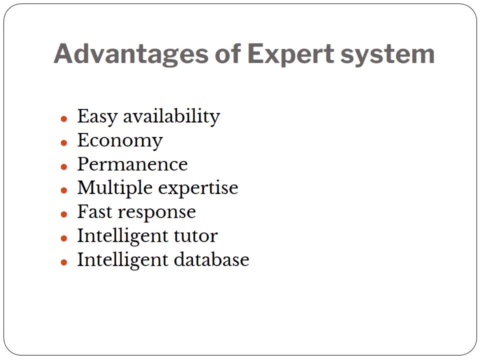 One expert system can be used in different places at the same time. Thus, the expert systems are tools of mass production. Human experts are not easily available and they have limitations of working hours. In addition, one expert can deal with one problem at a time at single play. 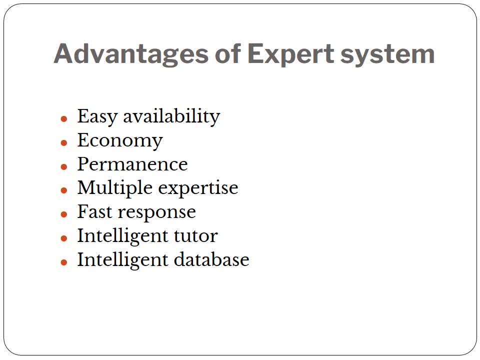 Next is the economy. Economy use of expert system is much more economical compared to humans. Next is permanence. The expertise of expert system is forever. Human experts may quit or die, but expert systems will last indefinitely. Next is multiple expertise. Multiple expert system can be used to work simultaneously on one problem and the combined expertise may exceed that of a single human expert. 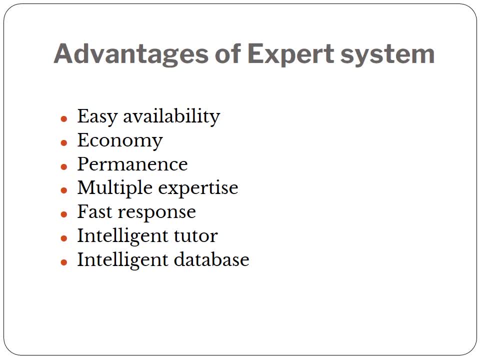 Next is about fast response. Expert systems respond faster than humans, depending on the hardware and software used in developing them. Next is intelligent tutor. Expert system can act as a tutor to someone who is interested in learning and reasoning, which is used in solving a particular problem by using the system for various examples. 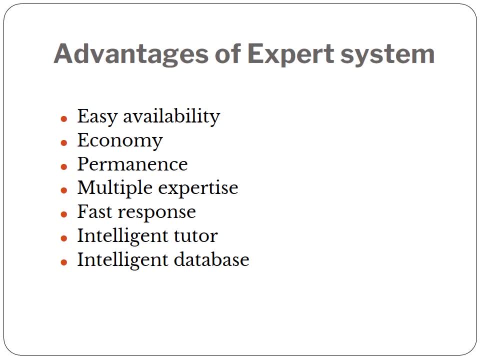 Next and last one is the intelligent database. Expert system can be used to access a database and the same can be used for some other purpose. So that's all about the advantages of expert system. So the next is about the architecture of expert system. 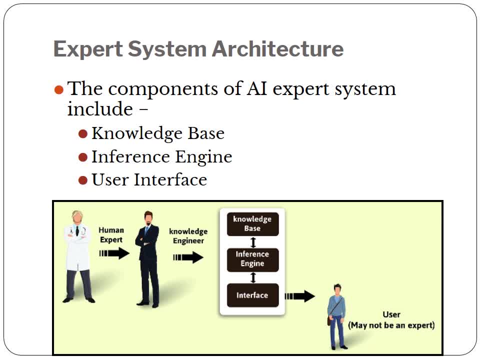 The main components of an AI expert system are Knowledge base, Inference engine. So, if you are considering the architecture, the interface is the one which the common man or the user will be interacting. The inference engine is the one that is interacting with both knowledge base as well as interface. 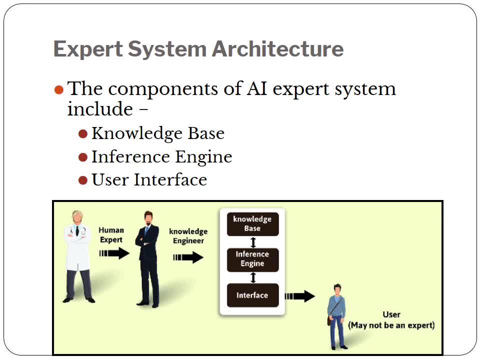 The knowledge base is the one that is storing all the domains of knowledge of the particular area, And the inference engine will be actually analyzing the knowledge that is stored in the knowledge base and it will be giving response to the user by means of the interface. 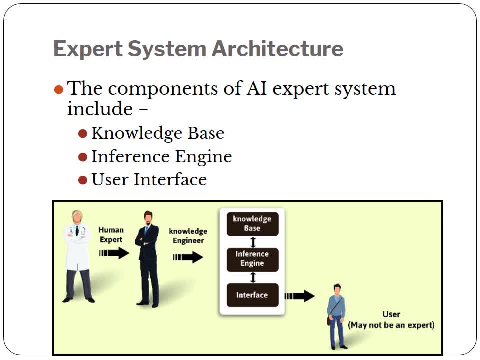 And the knowledge engineer, or the human expert, is the one that is handling the data inside the knowledge. He will be modifying, he will be coding and all these manipulations will be doing by the knowledge engine. Let us discuss each and every components one by one. 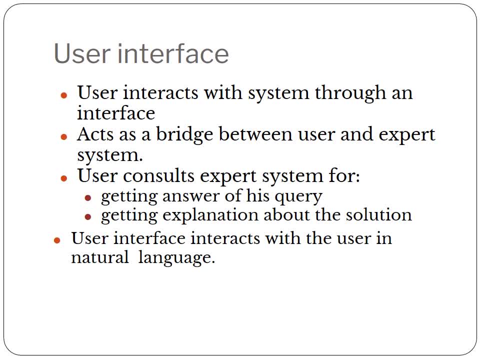 So, starting with the first component of rule based expert system, user interface. So user interacts with the system through a user interface. Mainly, we know what is the purpose of a user interface in desktop systems and all So similar to that. it acts as a bridge between user and expert system. 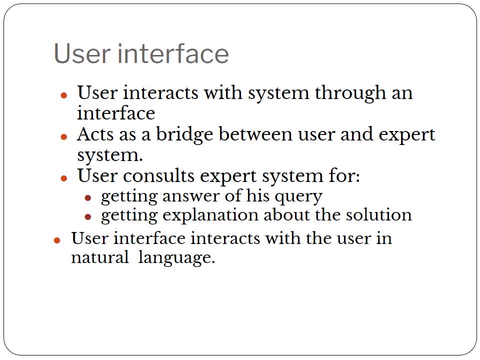 So this module accepts the user queries and submits those to the expert systems. So the user normally consults the expert system for the following reasons. First one is to get the answer for his queries and to get explanation about the solutions for the psychological satisfaction. 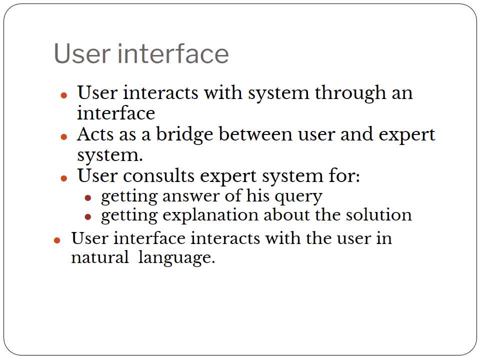 To make the expert system user friendly. the user interface interacts with the user in natural language, So presenting a real world problem to the system for a solution is what is meant by having a consultation. So the user interface provides as much facilities as possible, such as menus, graphical interface, etc. 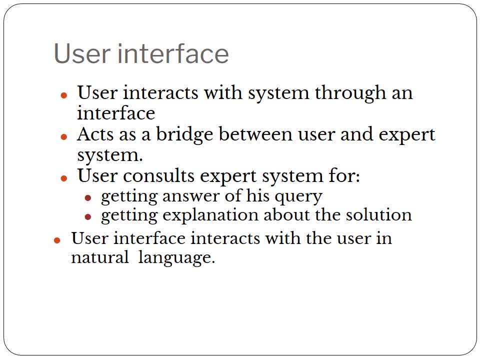 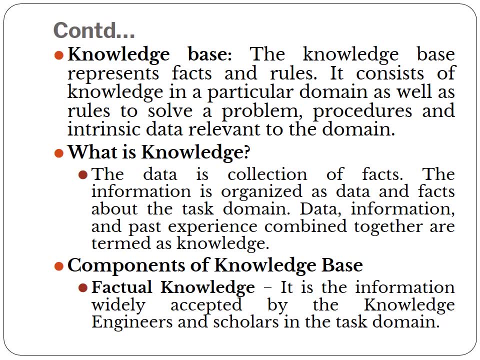 To make the dialogue user friendly and lively. So the next one is the knowledge base. So what do you mean by a knowledge base? So the knowledge base is the heart of an expert system. It is repository of knowledge in the expert system. 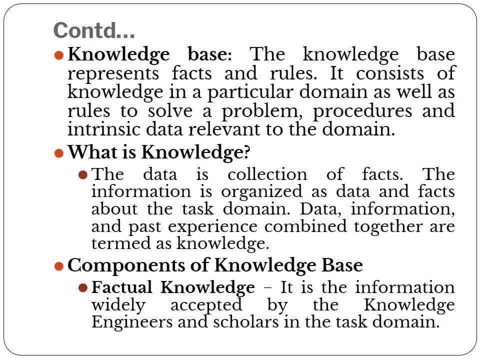 The expert system uses this knowledge to answer the queries or to give a consultation to the user. The knowledge base is a core module of any expert system. The capabilities of expert system are dependent on the amount of knowledge it contains. We require lot of knowledge to build an effective knowledge base. 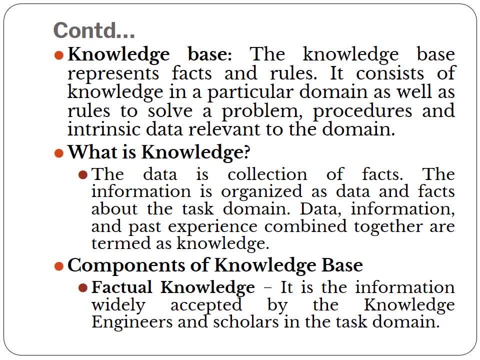 The knowledge is acquired from various sources by applying knowledge acquisition techniques. Knowledge acquisition is full-fledged area of research in the domain of AI. So what is a knowledge? The data is collection of facts. Similar to that. the information is organized as data and facts about the task domain. 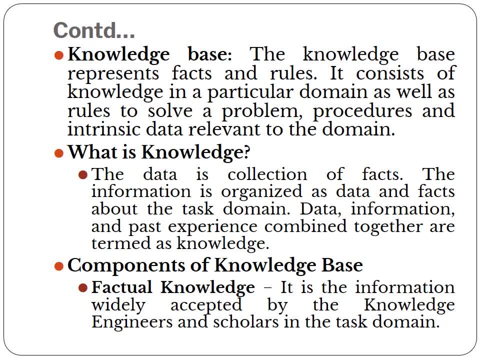 Data, information and past experience combined together are termed as a knowledge. So what are the different components of a knowledge base? So there are so many different components for knowledge base. One is factual knowledge. It is the information widely accepted by the knowledge. 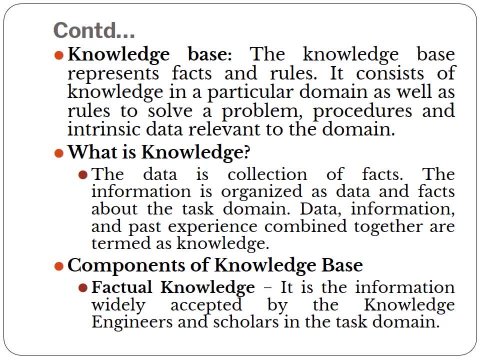 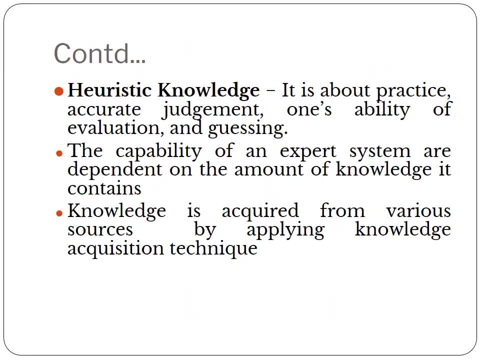 Like engineers and scholars in the task domain- So that is, the facts that are represented in a knowledge- is termed as a factual knowledge And heuristic knowledge. it is about practice, accurate judgment, one's ability of evaluation and guessing. So the knowledge that is dealing with these type of things are known as heuristic knowledge. 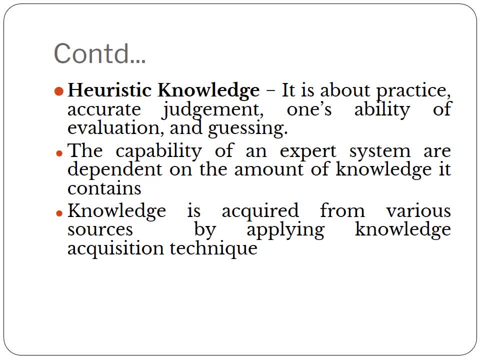 So the other types are also there, like common sense knowledge, task oriented knowledge and domain specific knowledge, etc. So the capability of expert system are dependent on the amount of knowledge it contains. We require lot of knowledge to build an effective knowledge base. 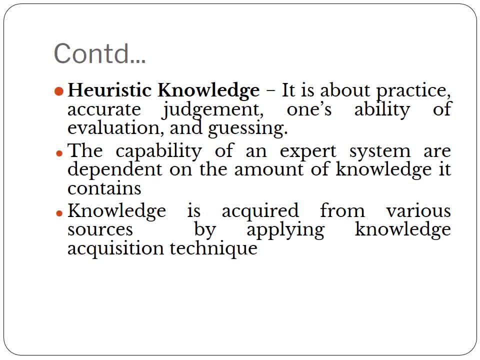 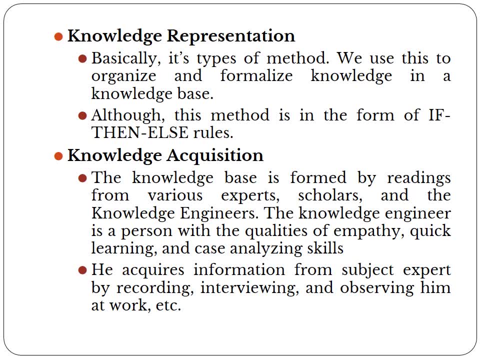 This knowledge is acquired from various sources by applying knowledge acquisition techniques. So the next topic is knowledge representation In inference to expert system. knowledge representation is mostly concerned with finding ways in which large bodies of useful information can be formally described for the purpose of symbolic computation. 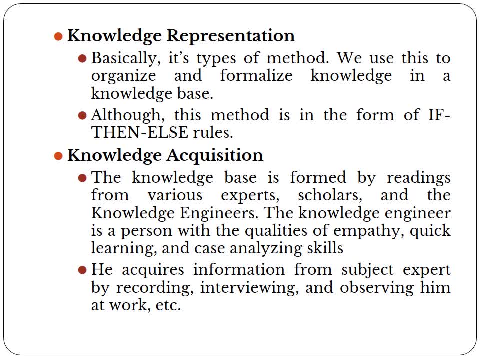 So basically, it is the type of method used for representing knowledge. We use this to organize and formalize knowledge in a knowledge base, So this knowledge representation will be normally in the form of if-then-else rules. So the next is about knowledge acquisition. 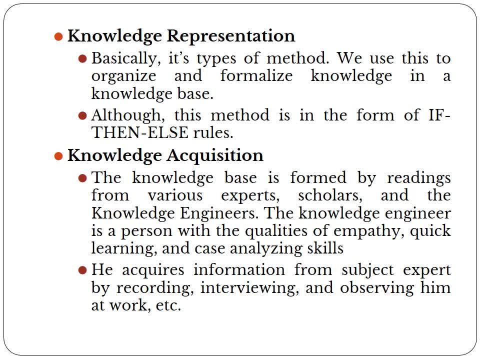 So different expert systems have adopted different methods for knowledge acquisition. So one is a compass method and so many different other methods are also there. So the knowledge acquisition is performed in the basis of the following steps. So the knowledge base is formed by reading from various experts, scholars and the knowledge engineers. 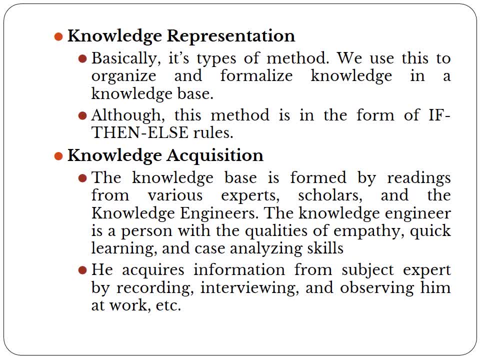 The knowledge engineer is a person with the qualities of empathy, quick learning and case analyzing skills. He acquires information from subject expert by recording, interviewing and observing him at work, etc. So we will check in the next slide what are the different steps for knowledge acquisition. 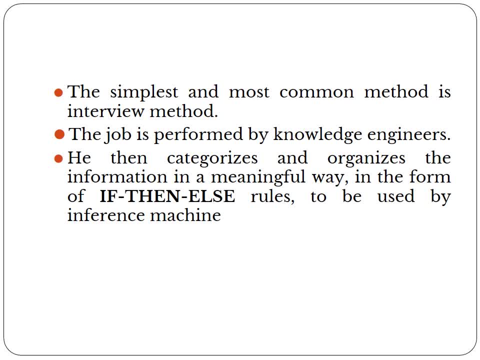 So the knowledge acquisition is itself a skilled job. The person interviewing the expert should also have some basic knowledge of the concerned field to find out what to ask. So the simplest and most common method is interviewing. This job will be performed by a knowledge engineer. 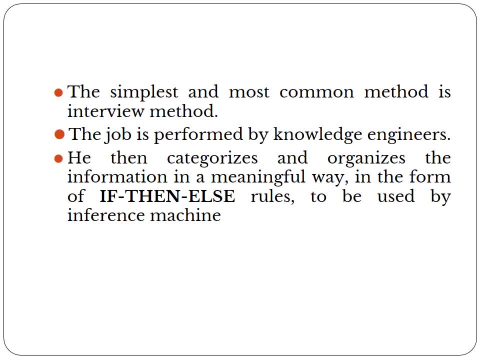 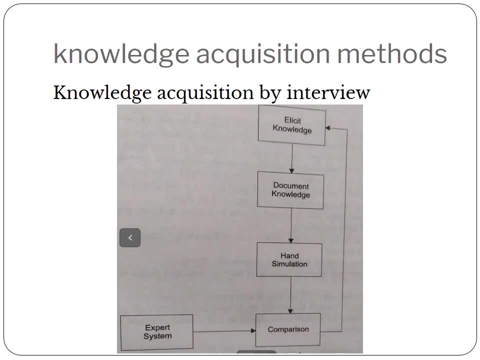 The knowledge engineer will categorize and organize the knowledge that is collected in a meaningful way. Normally it will be in the form of if-then-else rules, and this can be used by an inference engineer. So next is the different knowledge acquisition methods. 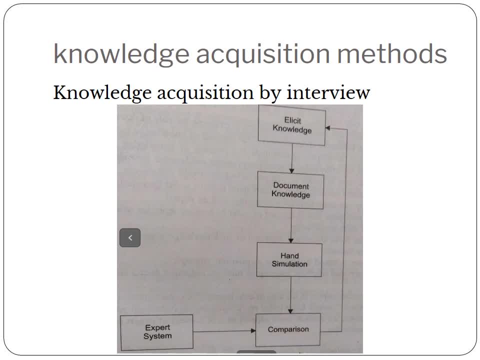 Different expert systems have adopted different methods for knowledge acquisition, So the first one is the knowledge acquisition by interview. The knowledge acquisition cycle performs the following steps during its functioning: It acquires the knowledge from expert documents, the acquired knowledge tests the new knowledge, as follows. 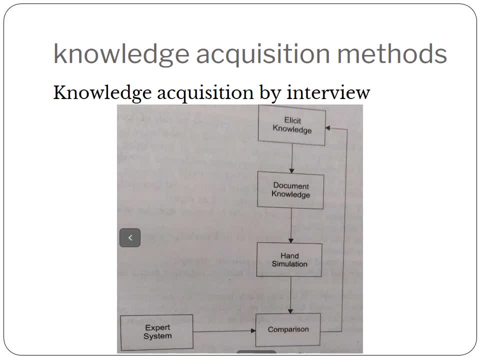 Exploits an expert to analyze the new state of data. analyzes the same data in the form of documented knowledge. compels the results of expert opinion. If the results differ, then finds the rules that generated the discrepancy and again starts from top to acquire new knowledge. 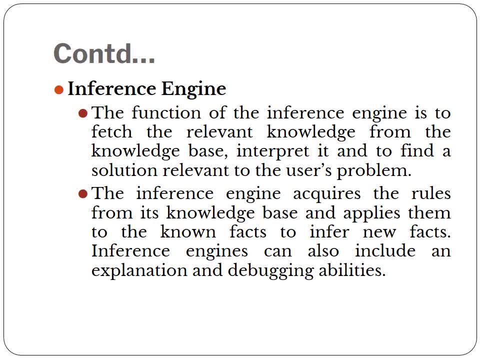 The next component in the architecture of expert system is inference engine. So what do you mean by an inference engine? So inference engine is the module which finds an answer from the knowledge base, Applies the knowledge to find the solution of the problem. 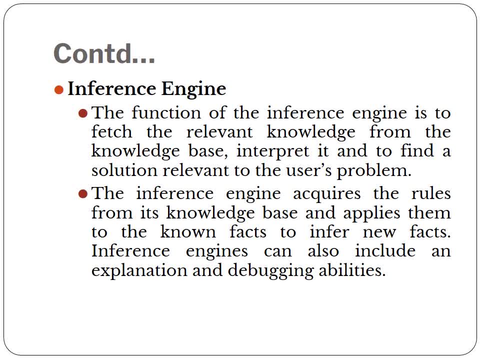 In general, inference engine makes inferences by deciding which rules are satisfied by facts, decides the priorities of the satisfied rules and executes the rule with the highest priority. It is also called rule interpreter, as the knowledge is normally stored in terms of rules, So the inference engine acquires the rules from its knowledge base. 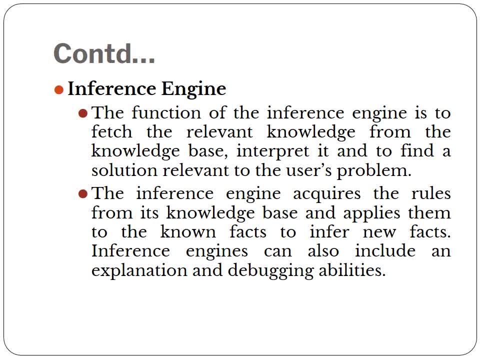 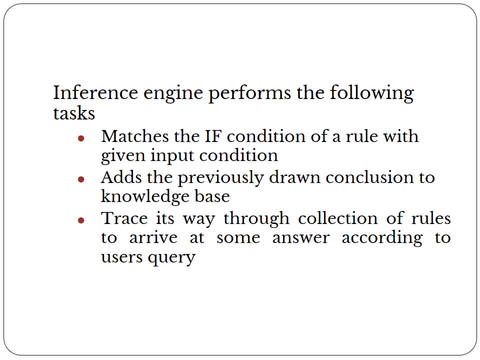 and applies them to the known facts. to infer new facts, Inference engine can also include an explanation and debugging abilities. So normally inference engine performs the following task: It matches the if condition of a rule with given input condition. If match occurs, then triggers that rule and similarly triggers many rules to reach. at conclusion, 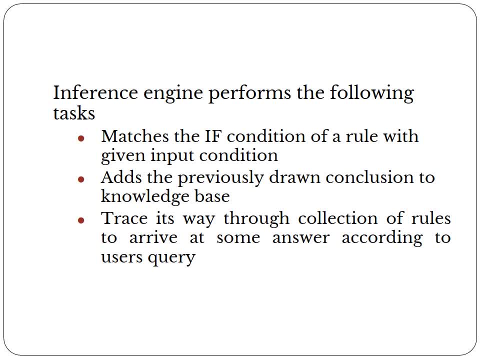 The second point is, as the previously drawn conclusion to knowledge base are inferred facts for future use, And the last and final task is the major task of inference engine. It is to trace its way through collection of rules to arrive at some answer according to usage query. 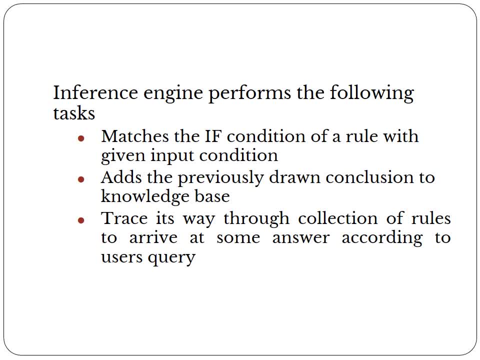 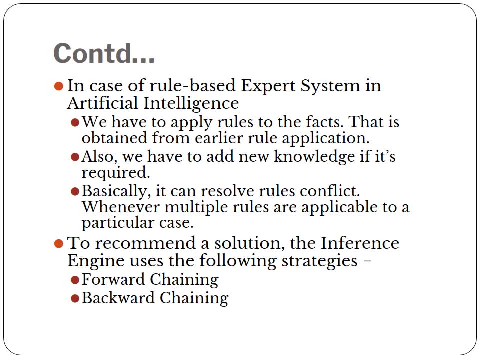 The technique of drawing the conclusion is known as inferencing. So the inferencing can be of mainly two categories: One is known as forward chaining and the second one is known as backward chaining. So in the case of rule based expert systems in artificial intelligence, as we discussed earlier, 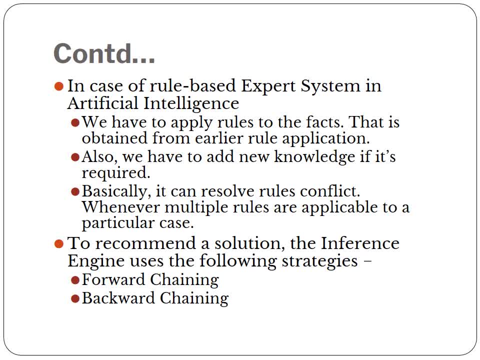 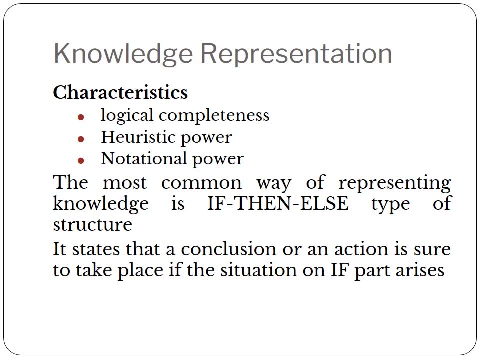 the inference engine should apply rules to the facts that is obtained from earlier rule application. Also, we have to add new knowledge if it is required. Basically, it can solve rules conflict whenever multiple rules are applicable to a particular case. So the next is another core concept of the rule based expert system about the representation of the knowledge. 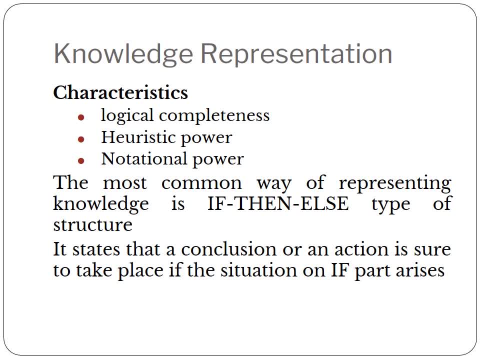 So the knowledge can be represented in some unambiguous language notation Which has well defined syntax governing the form of expression in the language And a well defined semantics which reveals the meaning of such expression by virtue of their form. The knowledge representation should have characteristics of logical completeness, heuristic power and notational convenience. 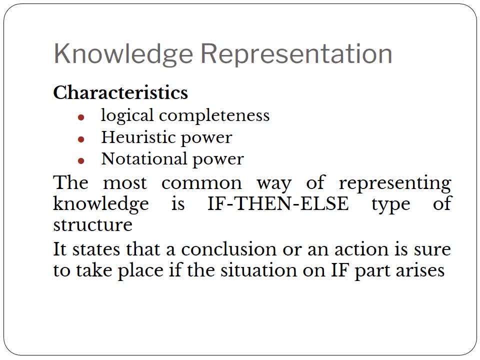 So what do you mean by a logical completeness? It means representation should be capable of making the complete description of the concept. For example, it is now possible to represent the idea that every drug has some side effect, unless one is able to differentiate between the designation of a particular drug and a particular side effect. 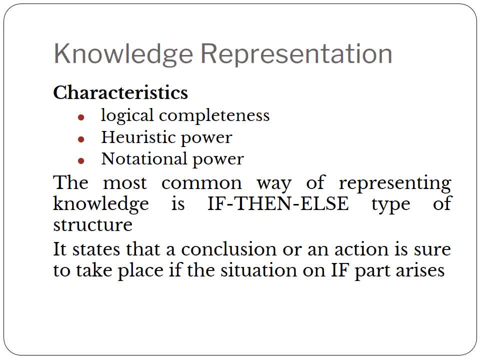 The next point is about heuristic power. It means that, though the representation should have a good expressive way, simultaneously there must be some way of using the representation to solve the problems in a short, straight format manner. The last one is the notational convenience, As the coding of vast amount of knowledge is required. 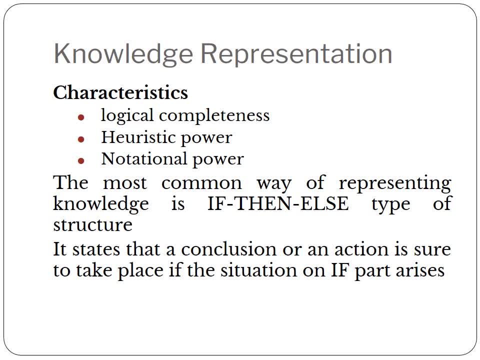 the notations chosen for coding should be easy to read and write, and it should be possible to understand the meaning without knowing how it will be interpreted. The most common way of representing the knowledge is if-then-else type of structure. So it takes or it states that a conclusion or an action is sure to take place. 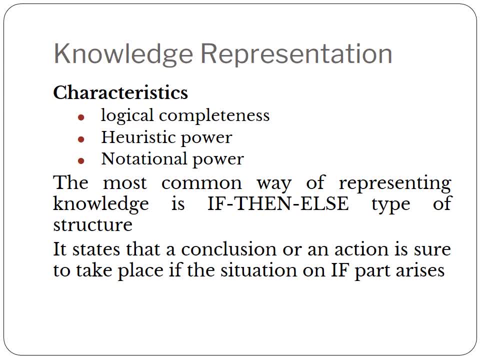 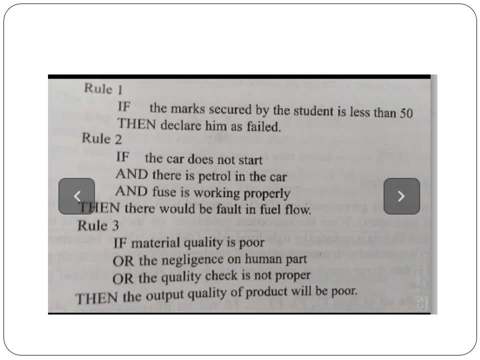 the situation or if part arises. So this is actually a form of rule. The first rule is indicating that if the marks required by the student is less than 50, then the action like declare he must fail should be taken. This is one type of a rule. 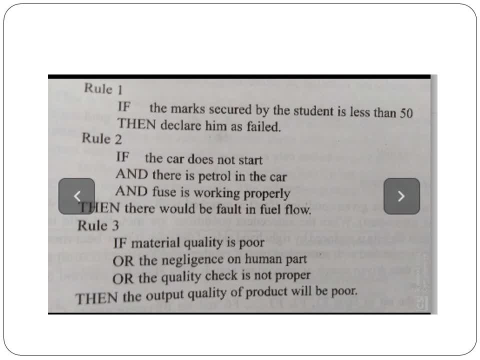 The second set is like this: If the car does not start and there is petrol in the car and fuse is working properly, then the action like there would be fault in fuel flow. So in the second rule type there are so many facts or two, three facts are connecting to this. 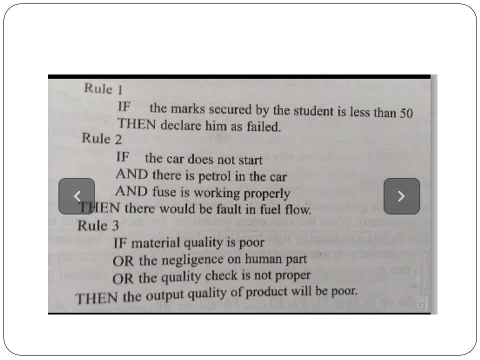 And the first one, there is only one fact. And the third one is if material quality is poor or the negligence on human part or the quality check is not proper, then the output quality of the product will be poor. So in the second one, AND is used, and the third one, OR is used. 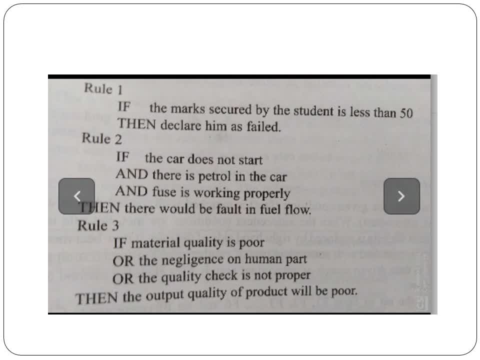 OR is used. you already know the property of AND and OR, So these rules simply indicate that each production rule is a fragment of AND or OR tree used for problem reduction. When I discussed about the production rule, When I discussed about inference engine, 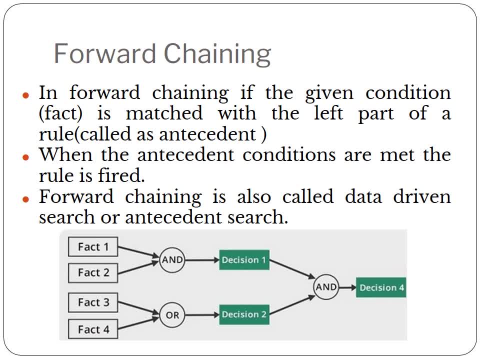 I mentioned about two types of inferencing. One is known as forward chaining and the another one is known as backward chaining. So let's check what are these. In forward chaining, the given condition, the condition is known as FACT And it is matched with the left part of a rule. 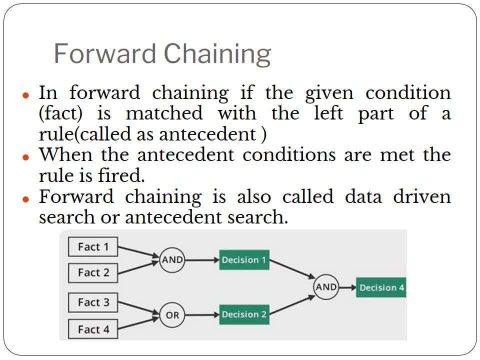 The left part of the rule is known as Antecedent. So normally if you are considering a rule, it will be having a left hand part and a right hand part. The left hand part is known as antecedent. So when the fact is matched with the left hand side of the rule, what will happen? 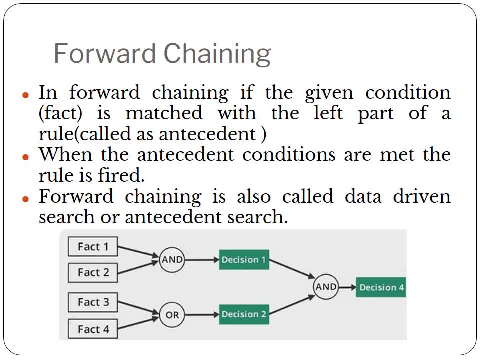 When the antecedent condition are met, the rule is filed. That means the rule is replaced by the right hand side of the rule. So it now becomes the new fact to be matched with the antecedent part of the another rule. That means the new one or the new replaced right hand side will become the matching condition for the next rule. 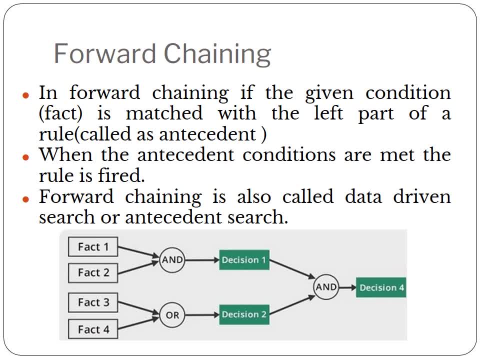 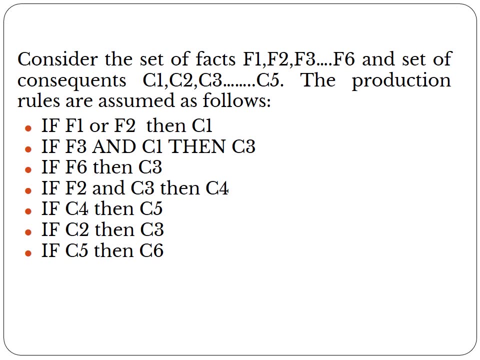 So the forward chaining can be also mentioned as data driven search or antecedent search. So the chaining will be the chaining method will be explaining in the coming slides. Consider the set of facts: F1, F2, F3, etc. up to F6. 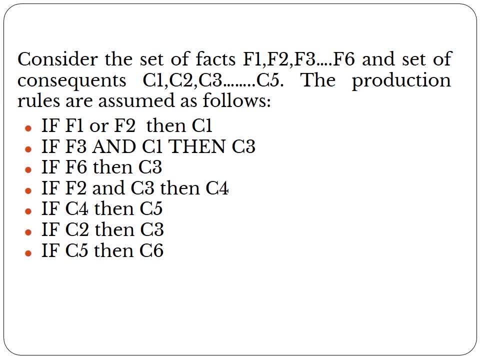 And set of consequence C1, C2, C3, etc. up to C5.. So we can assume a set of production rules. So the following production rules are: if F1 or F2, then C1.. If F3 and C1, then C3. 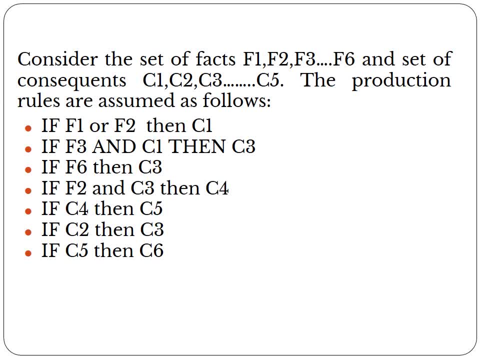 If F6, then C3.. If F2 and C3, then C4.. If C4, then C5.. If C2, then C3.. If C5, then C6.. So these are the set of production rules that we have. 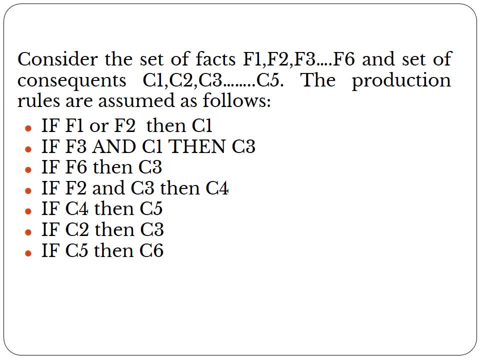 So let us assume that the input is facts F1 and F3.. So F1 and F3 are the inputs that we have and assume that F1 and F3 are true And the query is that we have to find out whether the consequence C6 is true or not. 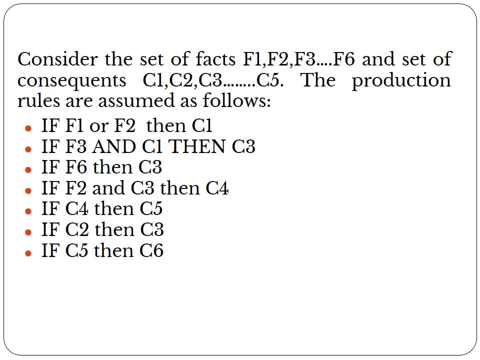 So how will the system proceed? So here we will be applying forward chaining. So in order to find out whether C6 is true or not, we have to start from the first rule, Because we have the facts F1 and F3 as inputs and it is given that they are true. 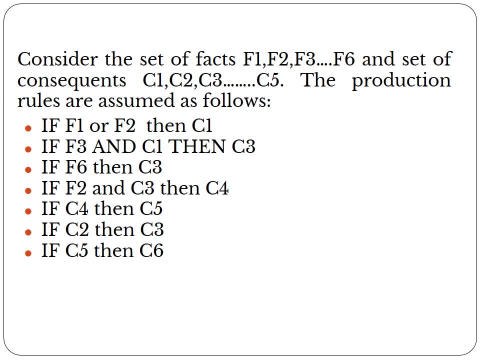 So upon checking the first rule, we can see that if F1 or F2, then C1. So we can infer that it is already given that F1 and F3 are true. So F1 is true, the condition that is given there is OR. 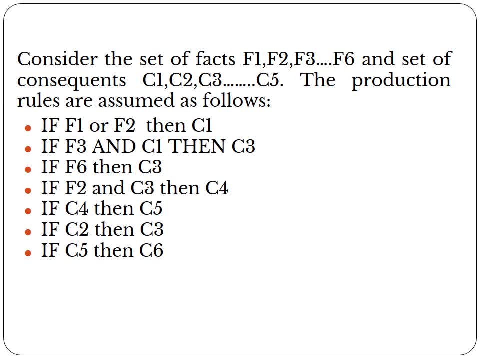 So we can definitely tell that C1 is true. So from C1 and F3, F3 is already given. So F3 and C1, here the condition is AND And F3 is given already and C1 we already got from rule number 1.. 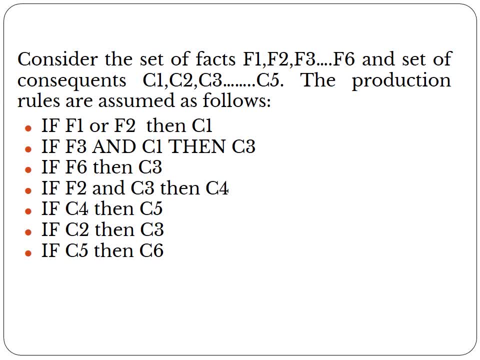 So, upon satisfying these conditions, we can assume or we can produce C3 as also, OR So, moving to condition number 3.. If F6, then C3. we already got in rule 2 that it is C3 is already true, So we don't need to again investigate rule number 3.. 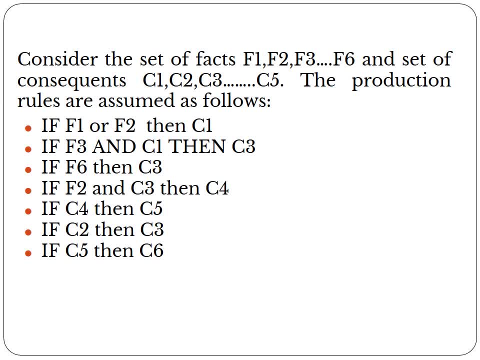 So we are not considering rule number 3.. So we will be directly moving to rule number 4.. So in rule number 4 we have C4.. So C4 is actually the combination of F2 and C3.. 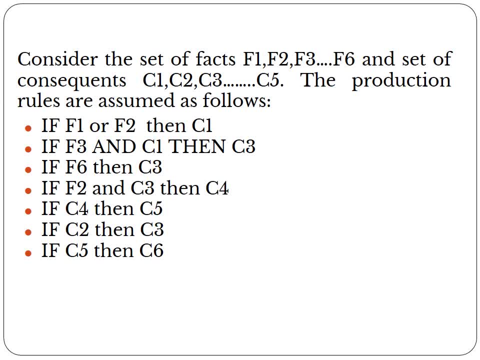 So F2 and C3, if you are combining them, we will get C4. So and C4 we need, because on investigating C4 or on assuming C4 as true, then only we can reach up to C6. So we have to definitely consider the rule number 4.. 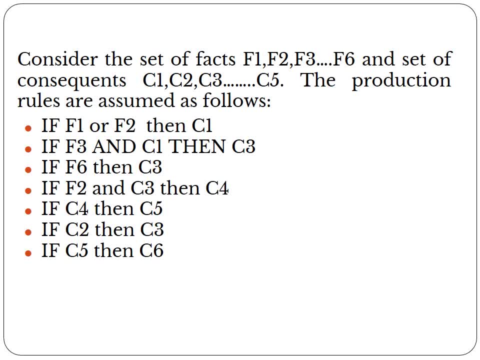 So if F2 and C3 are true, already we got that F2 is true and C3 is also true. So then we can produce C4 as also true. So upon moving to the next rule, that is rule number 5, it is given that C4 is C4, then C5. 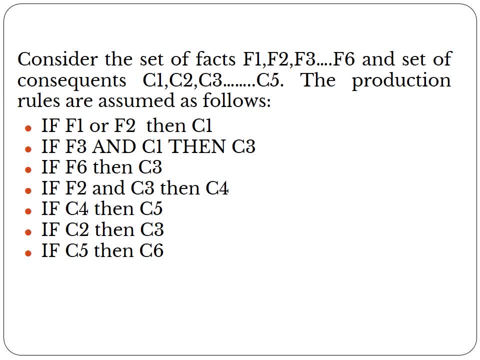 So we already got in the previous rule that C4 is true. So upon evaluating this one, we will also get that, or we can also analyze that C5 is also true. So again, the next rule is C. if C2, then C3.. 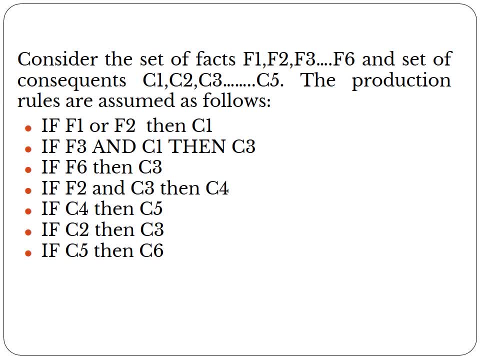 Here we don't need this condition because it is again going back to the previous one. That means C3. already we derived that C3 is true, So we are not going to consider that particular rule. So upon moving to the last rule, we already got from the previous 2, 3 rules that C5 is true. 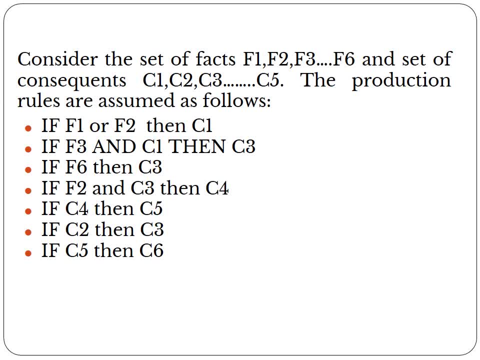 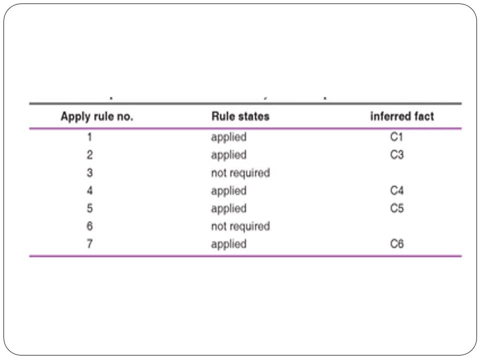 So C, C5, then C6. Like that we can reach to C6. So this is mean by this is the way for performing forward chaining. So this is the thing that I already discussed in the previous slide. So these are the rules: 1, 2, 3, 4, 5, 6, 7 are the rule numbers. 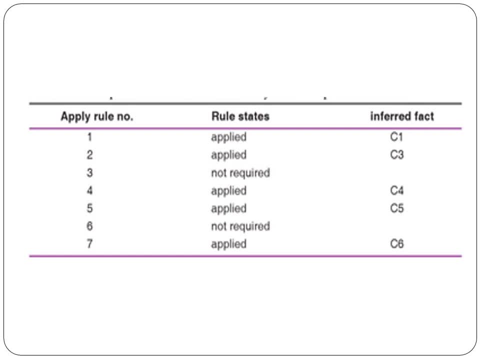 Rule states are there, whether it is applied or not applied, that will be indicated here, And the fact or the result that we will be getting in each and every rule or while applying each and every rule That is indicated in the inferred fact call. So we already I told you that the rule 1 you can apply. 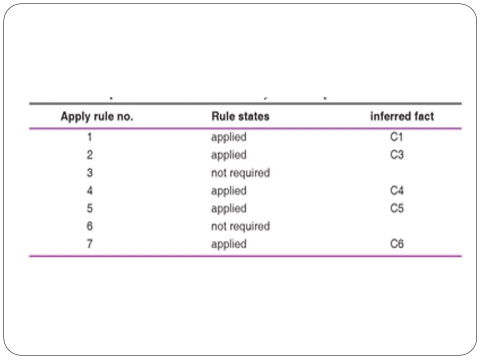 Rule 2 also apply, but rule 3 we are not considering here, So it is not required. Martha is not required. Then rule 4 and 5: it is also applied, Then rule 6: it is not required, Rule 7 applied and we will be getting the final result. 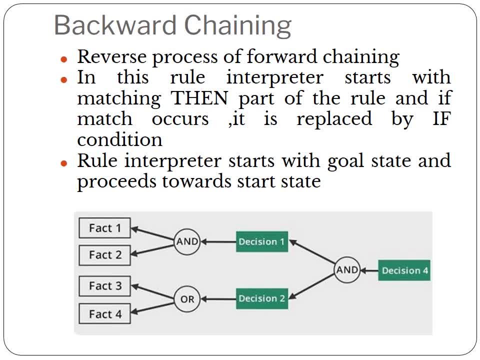 So this is known as forward chaining. The next one is backward chaining, So backward chaining. So this is the reverse process of forward chaining. In this rule, interpreter starts with matching, then part of the rule, and if match occurs it is replaced by if condition. 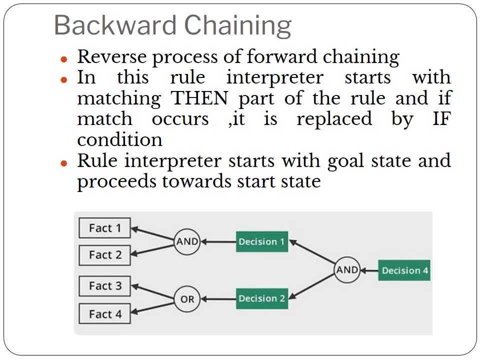 Here the rule interpreter starts with the goal state and proceeds towards the start state. Thus backward chaining is also called as a goal driven search. So here we will be moving from the goal state to the initial state. But in the forward chaining method we derived the goal state from the initial state. 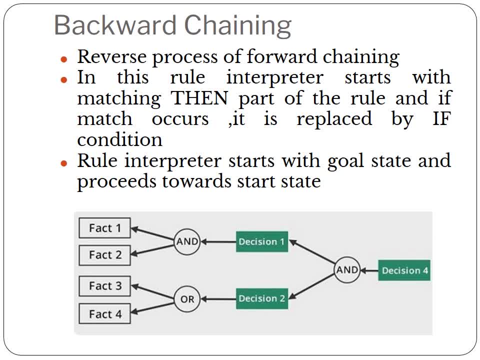 And in the backward chaining method we will be moving from the goal state and we proceeds towards the start state. So this is the main difference between forward chaining and backward chaining. So, moving again to the next example, So let us discuss an example for backward chaining. 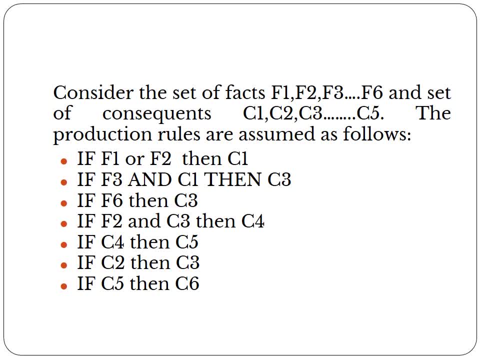 Here we are having the same data or the same example that we discussed for forward chaining. So consider the set of facts F1, F2, F3, etc. upto F6 and set of consequence C1, C2, C3, etc. upto C5. 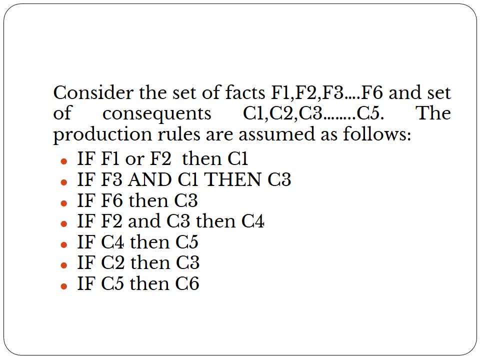 So assume the production rows given below. So we have C6 as the consequence. that is already given and we are assuming that C6 is true. And also we are assuming that F1 and F3 are true and we need to find out F1 and F3 from C6.. 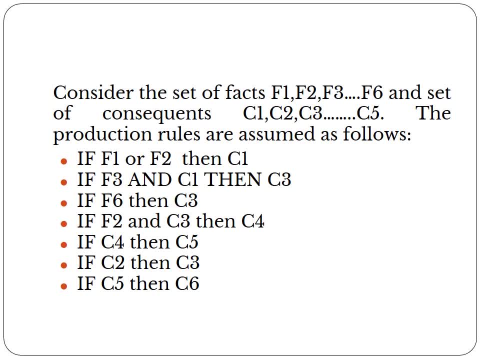 So in the last rule it is given that if C5 then C6. So from the rule we can assume that from C6 we can derive C5. So, and moving above, we can derive C4 from C5, and again we can derive C3 and F2..